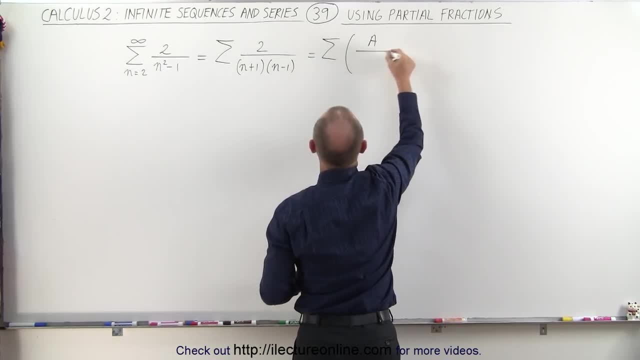 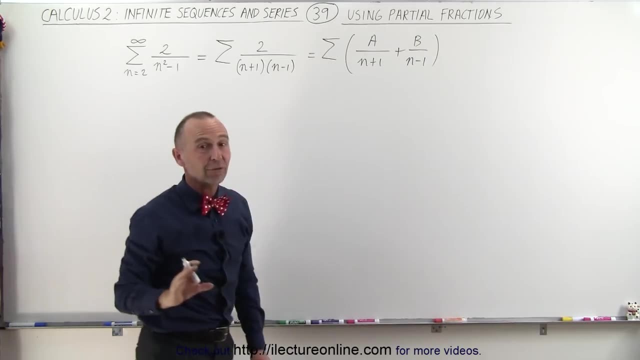 sum of a divided by n plus 1, plus b divided by n minus 1.. And then we use the technique of partial fractions to solve for a and b, and then we can sum up the two infinite series separately. So how do we do that? 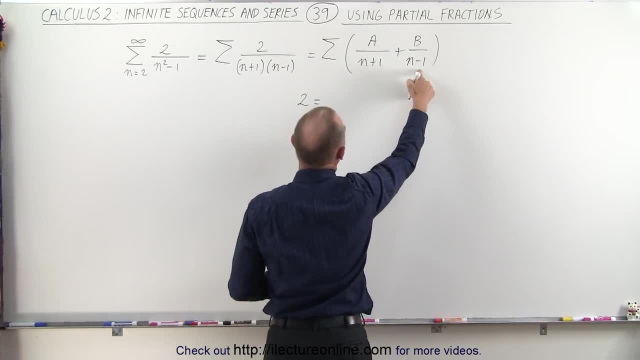 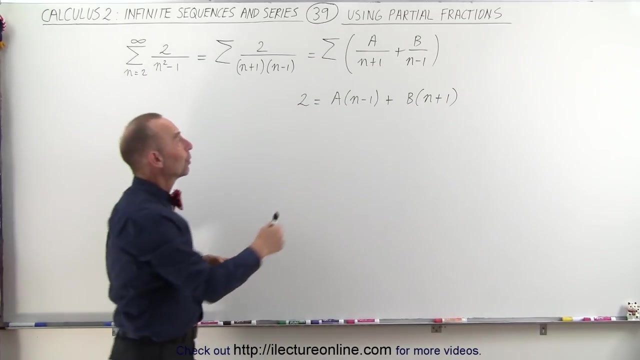 Well, we can say that 2 is going to be equal to when we multiply a times n minus 1, plus when we multiply b times minus 1.. Oh, I should say b times n plus 1.. What we're actually doing here is we're writing this. 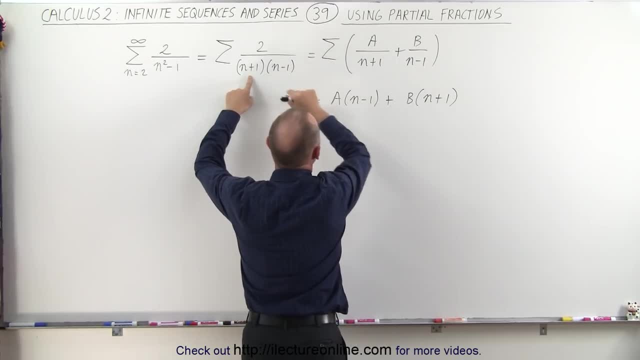 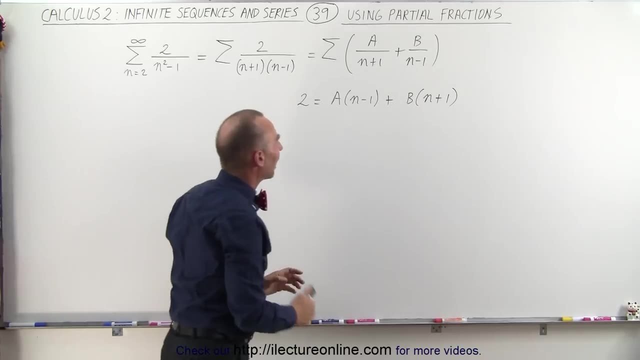 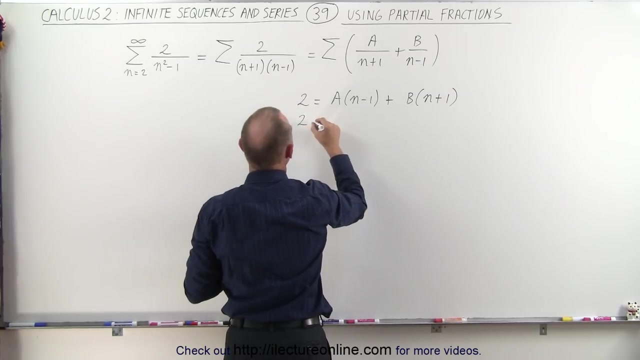 over a common denominator of n plus 1 times n minus 1, which means that a times n minus 1 plus b times n plus 1 has to equal the numerator of that. Now we can solve this for a and b. Notice, if we write this out, we can say that 2 is equal to a times n minus a plus b, times n plus b And for: 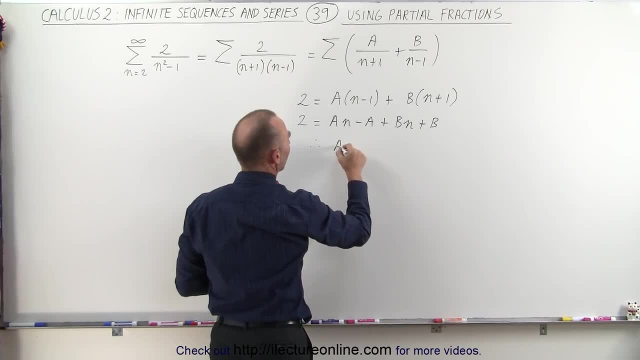 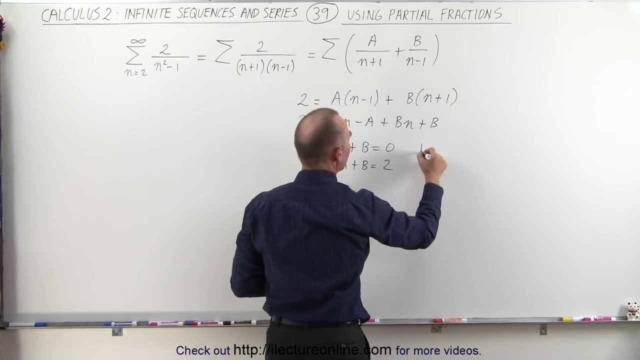 that we can conclude that a plus b must equal 0, because there's no n counterpart on the left side of the equal sign And we can say that minus a plus b is equal to a. plus a is equal to minus a. So that means that b is equal to minus a and if I plug that in here, we have: minus a minus a is equal to 2. she comes back with 2 times A. 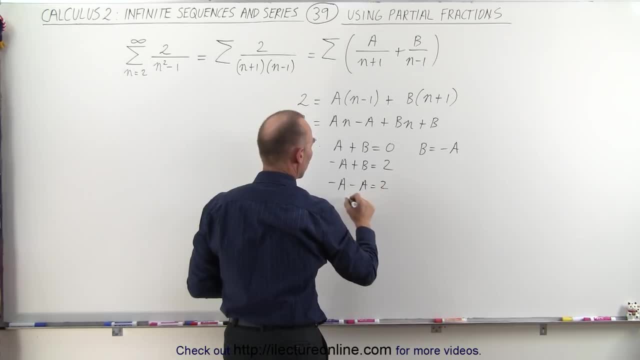 is equal to 2.. Or a is equal to minus 1.. So timelands get area wars. with respect to the inverse, leave the Aussie w regulams. in that I leave the term I E poser a and I'm going to put uh, m employer's law and that's a where an S gives me the 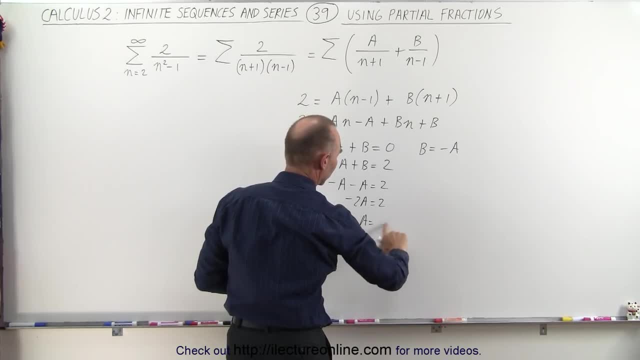 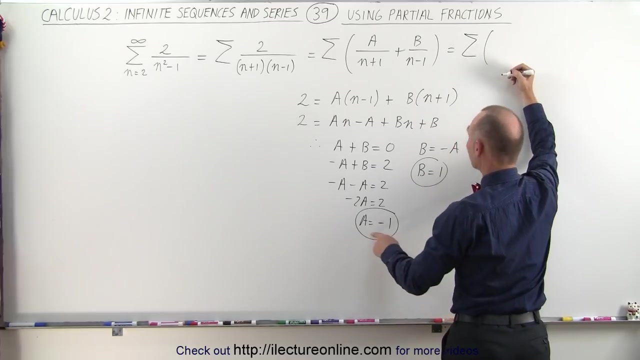 a is equal to minus one- oh, i didn't write that right- minus one. there we go. so if a is equal to minus one and b is negative a, that means that b is equal to one, which means that this can now be written as: the infinite sum of a, which is minus one, minus one, over n, plus one plus b, which is one. 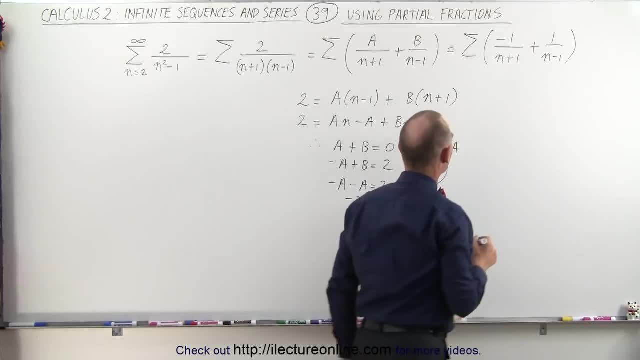 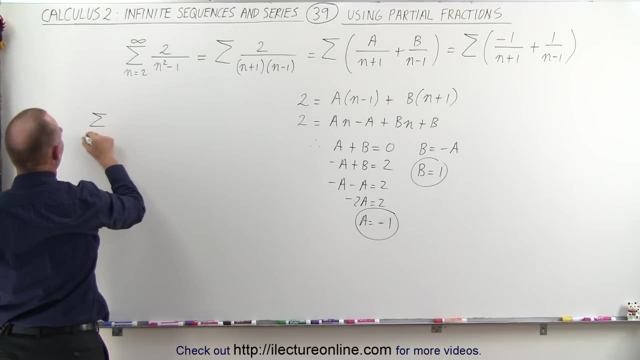 over n, minus one. all right, so now we're going to sum those up separately, and so we're going to get the sum, as n equals two to infinity, of minus one. divided by n plus one, this is going to be equal to starting with the first one. if n is equal to two, we get minus one over three, minus one over four.